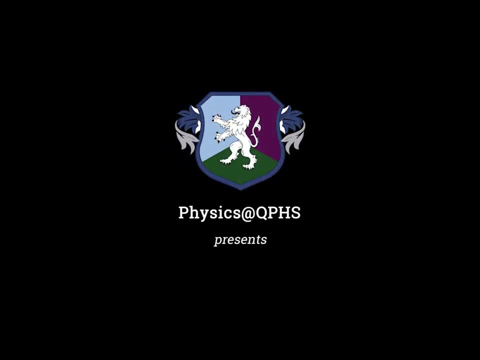 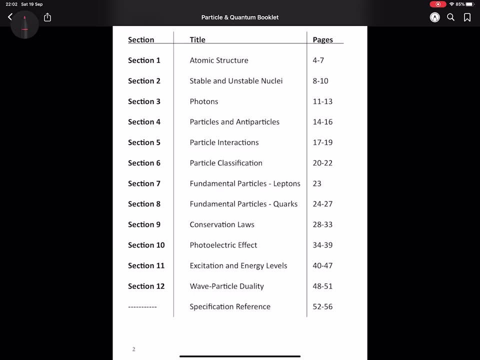 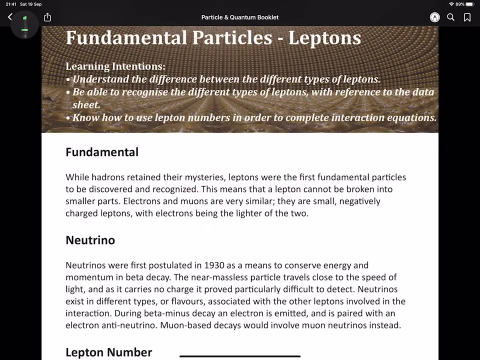 In this video we will be looking at the first set of fundamental particles: leptons. Now, moving on from the crazed particle zoo we were just introduced to, we now can look at the first fundamental particle that was discovered and largely ignored: leptons. Now, 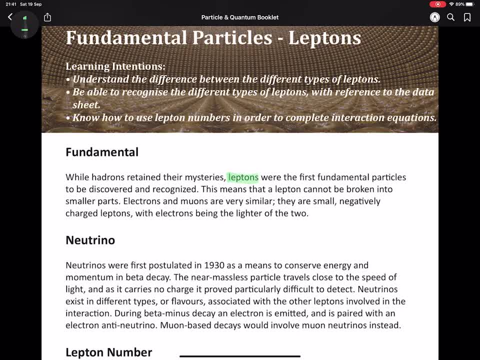 electrons and neutrinos fell into this category and they were fundamental because they could not be broken into any smaller parts. Now a larger version of the electron was also discovered, known as a muon, given by the mu Greek letter, And they're very similar. 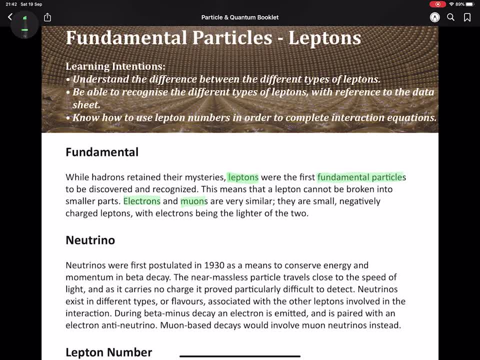 the muon is just a slightly larger version of an electron. Now neutrinos were the more challenging aspect, as for a long time they were just theoretical and existed again as a conservation of momentum, so a balancing factor in equations, Now being near massless and having no charge and also travelling near the speed of light. 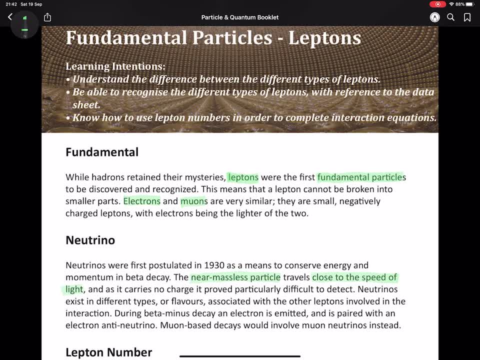 made these seem absolutely unrealistic. But eventually, through incredibly large detectors deep underground or under layers of ice, it was possible to finally notice some interactions that involved leptons Neutrinos travelling from either reactors or from space. Now neutrinos, as a mathematical fix, have a key identifier that distinguishes different. 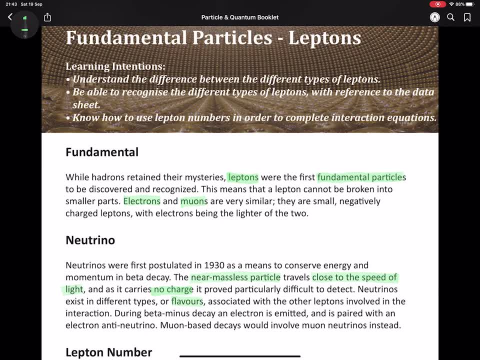 types of them. Now, instead of repeatedly using the word type for particles, we instead, at this point, can use the term flavour. So in an interaction that involves electrons as their key lepton, Any neutrino or antineutrino will have a little e written next to it, making it an.